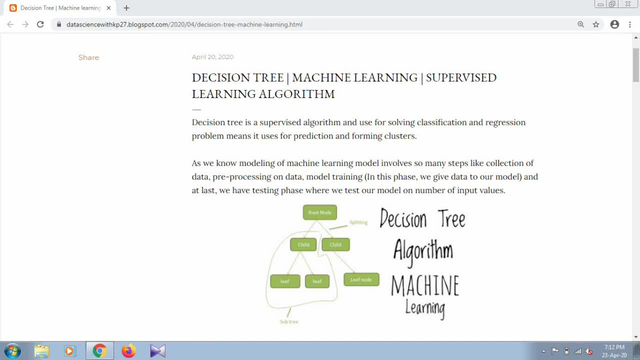 values. suppose we have a data set which is related to the different different shapes and geometrical shape like a circle, a square, straight line, etc. and we have to classify our model like this that we have at last we have a separate clusters, like one cluster is also only having the circles, one classical clusters, at last only. 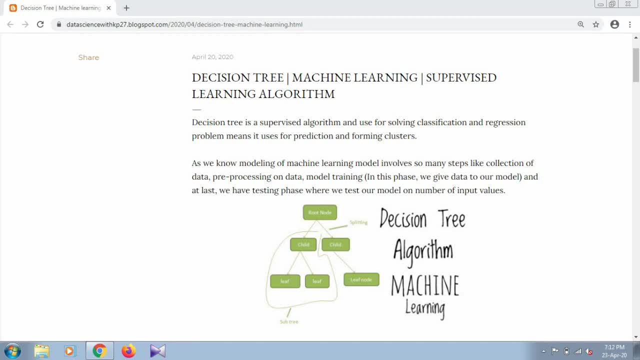 having the square and one cluster is only having the straight line. and this is the classification problem. and what is the recreation regulation is nothing but the predicting a value, predicting a value of variable that is depend on the another variable. or we can say another feature like: suppose we have two. 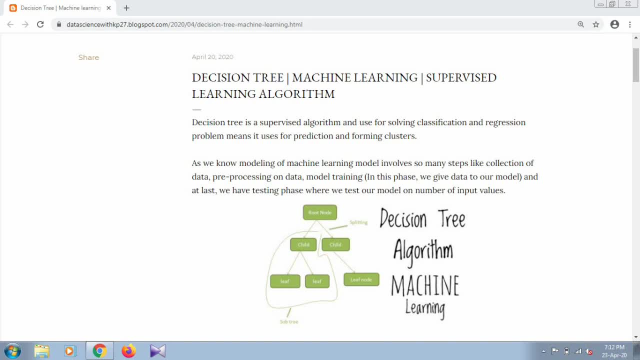 variables X and Y, where Y is the salary and X is the experience in year. so we have to predict the what salary will be according to the experience in years. so this is all about the regulation problem. so, as we know, modeling of a machine learning model involves so many steps like collecting of data, pre-processing, 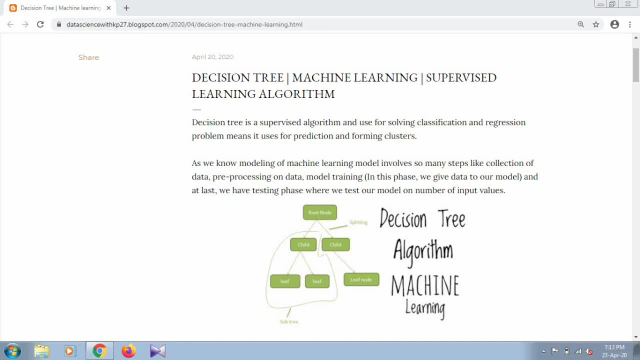 on that data model training. where we have to, we are, we split. we have used train and test technique for splitting our data into the sum. ratio means one: one data is used for the testing and another is used for the training. so this is all about the training model, training in the more. 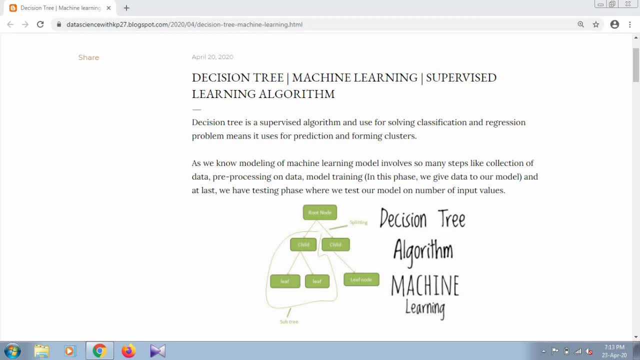 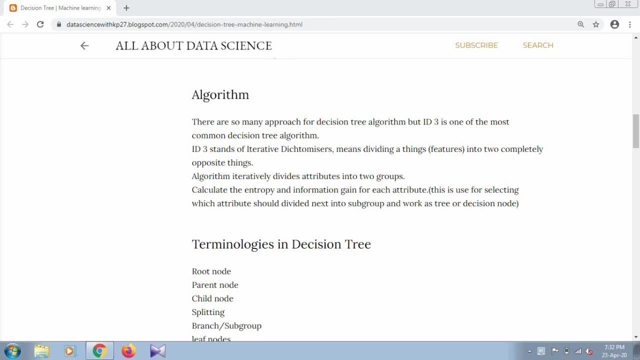 amount of data we will give in a training phase, the more accurate will be in the desert. okay, so this is all about the decision tree algorithm. now see the algorithm for the decision tree. there are so many approaches for the decision tree algorithm, but ID 3 is one of the most common decision tree. 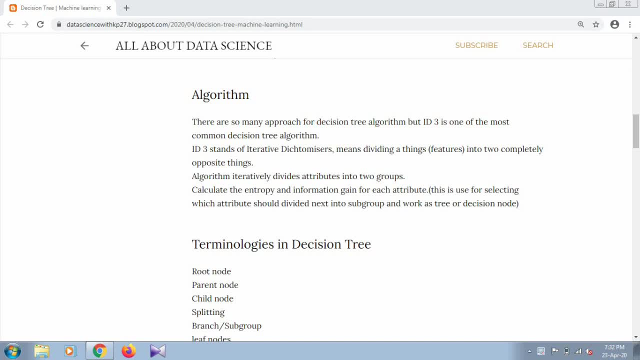 algorithm. ID three is 10, for the iterative determine means dividing, I think, into two different, completely different opposite things. there is the algorithm iteratively divides attribute into two groups and we select that group for the further splitting process has less number for entropy or we can say the highest number of information gain. we can also select the by: 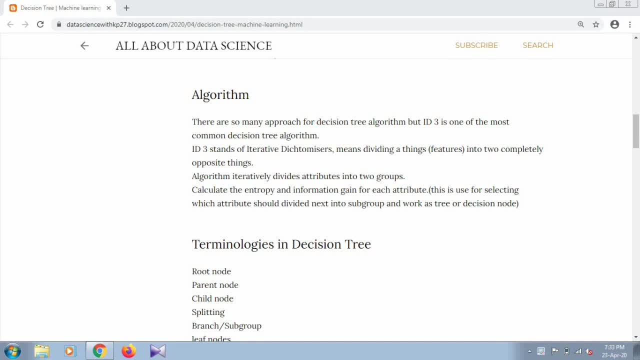 get the maximum amount, which is equals to the information gain minus entropy. so this is all about the selecting: how to select an attribute that is going to be further divided, or we can say further splitting. okay, so this is algorithm for the decision tree. now go for the terminology that is related to the 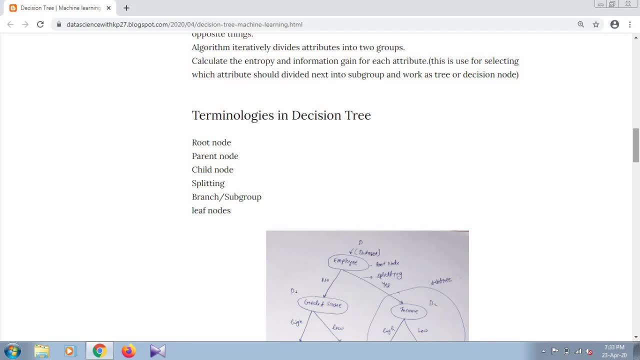 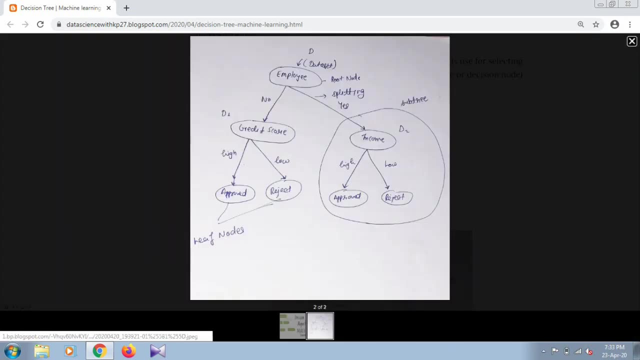 decision tree. basically there are three, four and five terminologies are there. that is root node, parent node, child node, splitting branch, and the leaf nodes- we can say decision nodes- are also there. decision nodes are nothing but the node that is responsible, or we can, that is responsible for the further splitting. 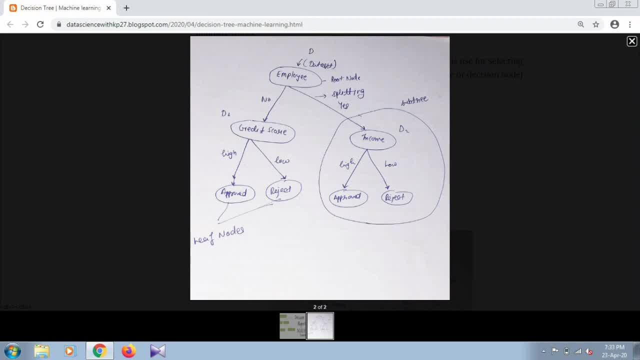 we can for the decision, okay. so here's the example. here we we have a data set of the person, some of some of them are the employed person, some of them are the unemployed person, and we want to predict whether and if any person know and will be rejected or approved. okay, so we have to start. we give, we. 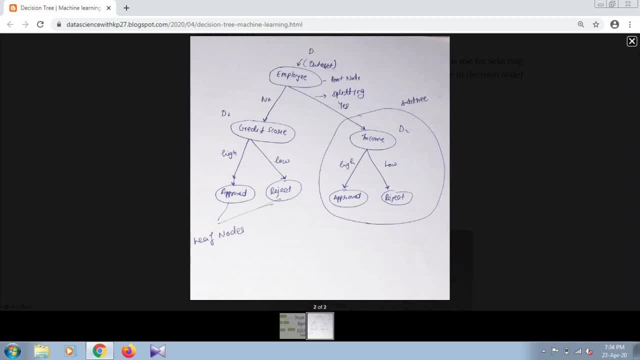 take the data set of the person and we take the data set of the person and we take our whole data set and split our data set into two parts: one for the employed person and another for the unemployed person. so this is our data set imply: if the person is employed, then it will go for the yes, and if the person is 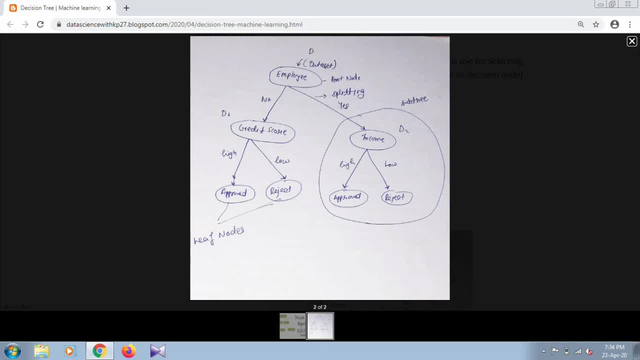 not employed, because they are unemployed and it is go for the no, okay, but if the person is employed, then we will check their income, okay. so this is the. this is the whole data set D, and now we are dividing our data set D one, that is that: 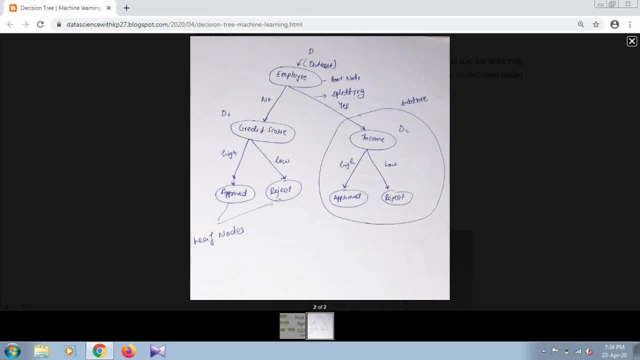 data set that person is unemployed, and D two on those person who is employed. if the person is employed, then we will check the income of that person. okay, it the income is high, then we will simply approve your loan. if the income is low, then we will reject the loan. same for a kid. if the person is unemployed, then we 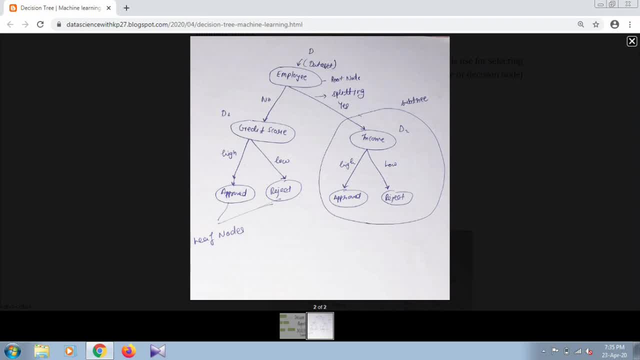 will check their credit scores. in that credit score is high, then we will approve the loan of, otherwise we will deny. okay, so this is all about the working of a decision tree algorithm. and, and, for the terminologies imply, is the highest node of our tree. so this is the. this is the root node of our tree. okay, 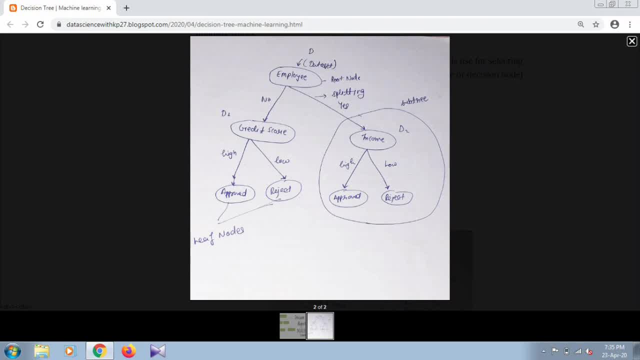 and it is also works as a parent node for that credit score and income. credit score and income are the child node of the employee, but credit score is the parent for the approved and the reject, and income is also parent node for the approved and reject, and here approved and reject are the leave nodes on both. 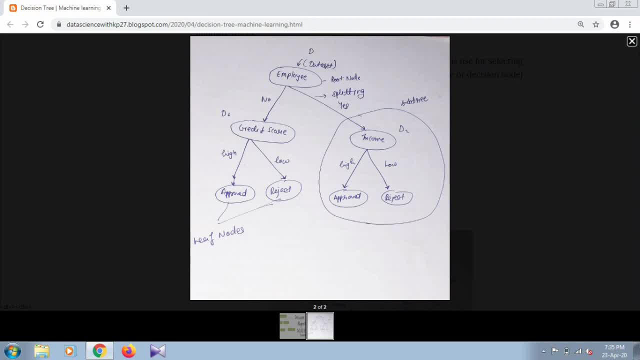 sides okay. and what is a decision node? actually, decision node are nothing, what the node that is for the splitting, or we can further provide any decision. so here, Caryly score and the income are the two decision node, as it is responsible for the weather the loan is approved or reject. so credit is coarse and income 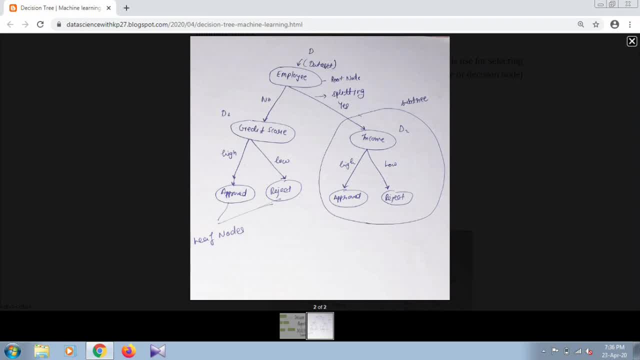 at decision node for this tree and one other terminal terminologies are there, that is subtree or branch. okay, so income approved- reject. or we can say category score approved, reject. it work as a subtree, subtree, subtree or nothing but a tree which is inside a complete tree. we can say inside a tree which is satisfy all the. 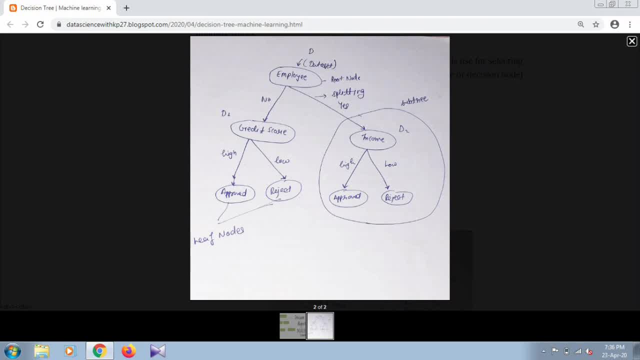 requirement of being a tree. suppose there is a. now I am checking whether this subtree is satisfy all the requirement. yes, I will checking income. this is a root node for this subtree, this is the child, this is a parent and this, these two arrows shows, are splitting. so yeah, these two, these, this, 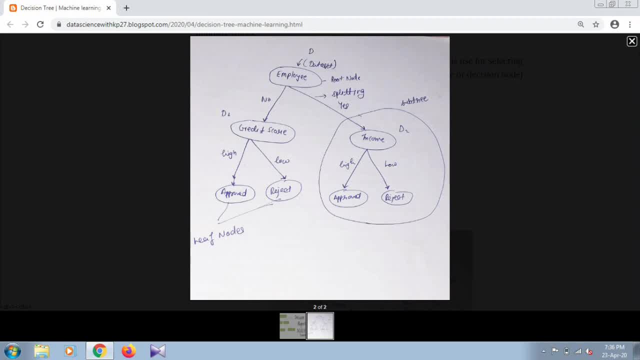 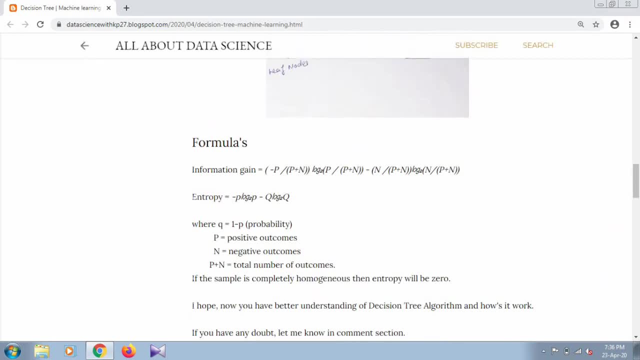 is a subtree, or we can say branch, of this whole node. so this is all about terminologies and the working of a decision tree algorithm. so this will be discussed. so, formula: how will calculate the information gain and entropy? so this is the formula for the information gain and this is entropy, and 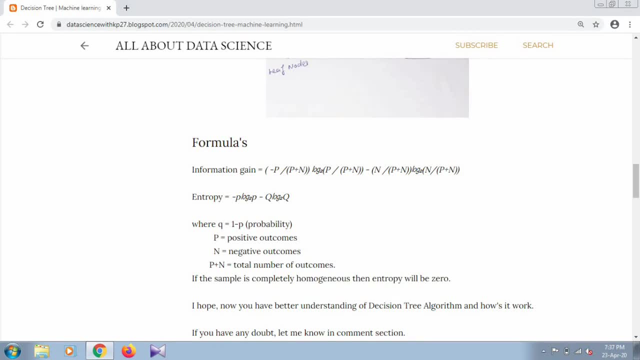 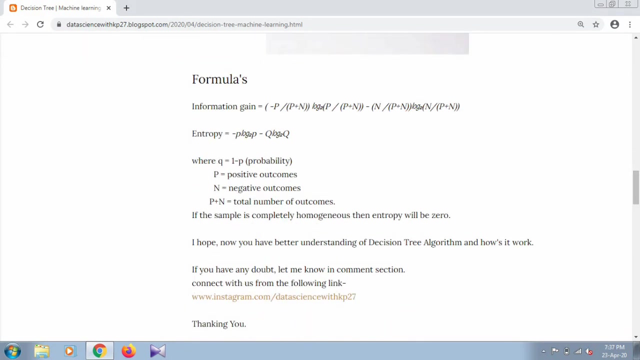 here the terminologies that used for the in the formula, that is, P is nothing but a positive outcomes and is the negative outcomes. Q is the probability for not happening anything. that is 1 minus P. P is the probability for happening something and P plus and the total number of observation. we can say total. 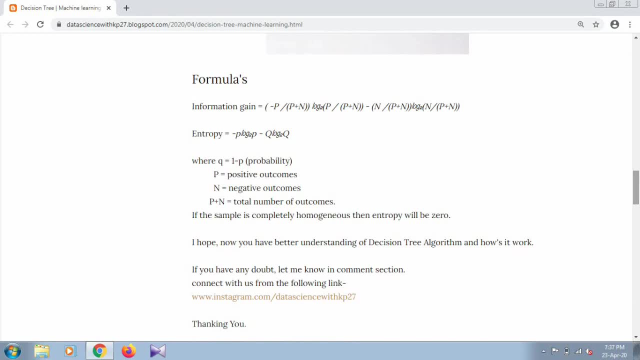 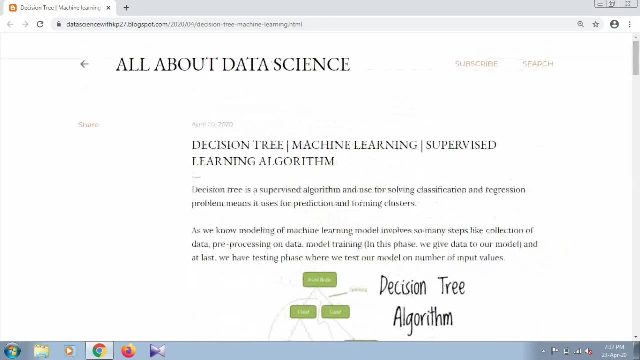 number of outcomes. okay, so this is all about the decision tree algorithm. so if you have any doubt, just drop a comment, and if you want the whole documentation of this algorithm, just check the description. I will provide a link. so thank you for watching this video, you, you. you, you, you, you you.